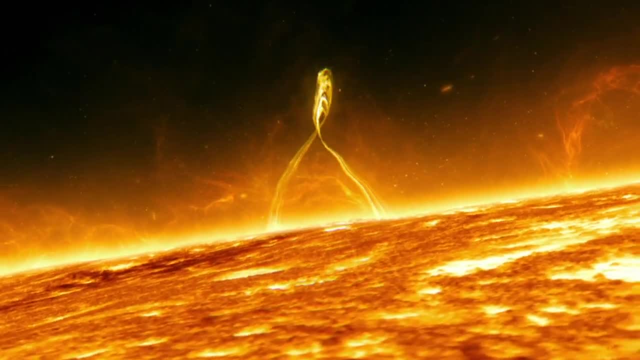 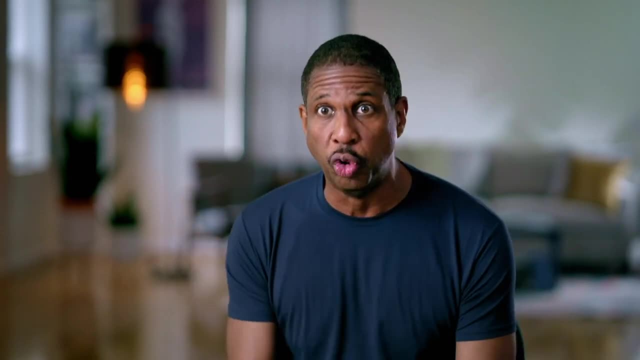 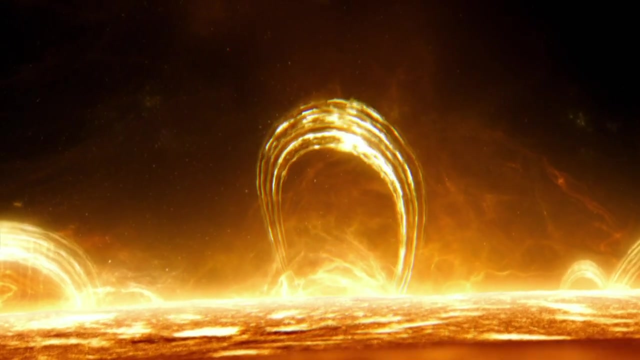 When the magnetic field lines snap, energy bursts out, And sometimes that energy release is explosive, And that's what results in flares, which are these huge bursts of light. The probe discovers that after a solar flare, the Sun's surface stores electrically charged particles. 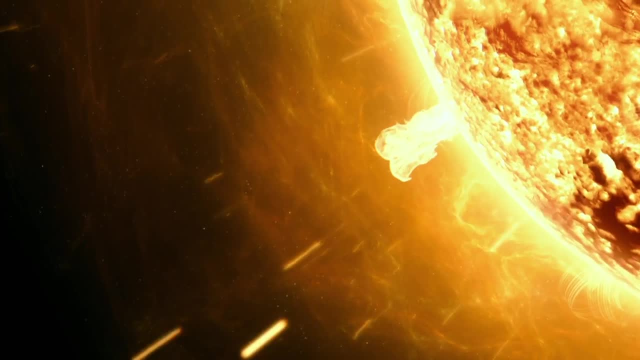 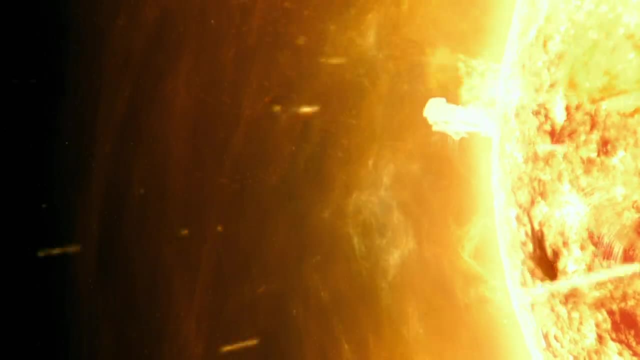 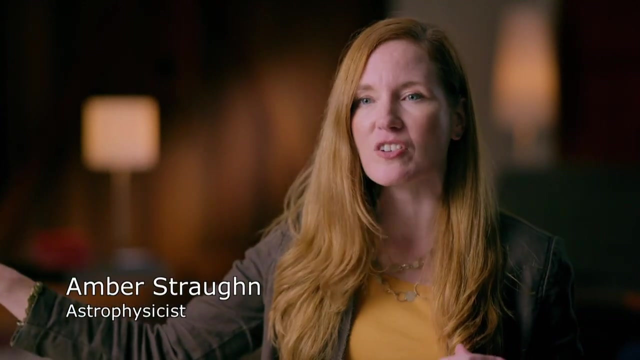 But sometimes there's a second explosion called a coronal mass ejection, releasing superheated electrically charged gas called plasma. These giant balls of plasma go flying off the surface of the Sun And in those balls of plasma are contained these charged particles. 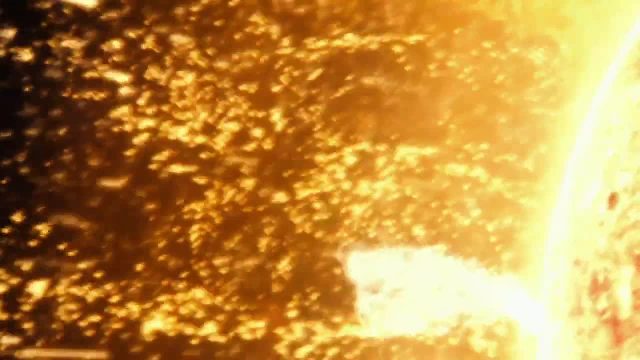 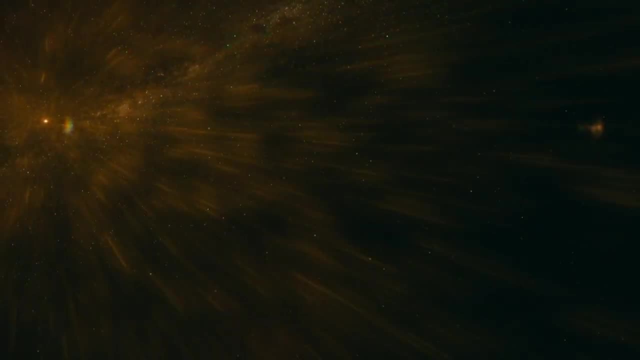 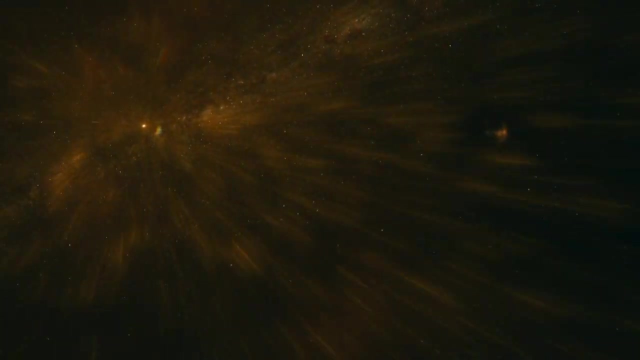 The charged particles move fast, But they hit a roadblock, A cloud of slower-moving particles that always surrounds the Sun, The solar wind. Well, the coronal mass ejection is moving into the solar wind much faster than the wind is moving. 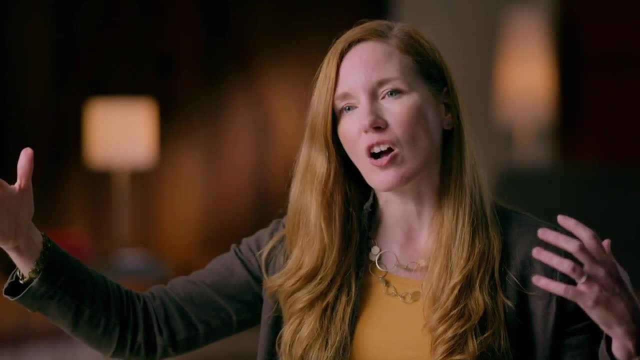 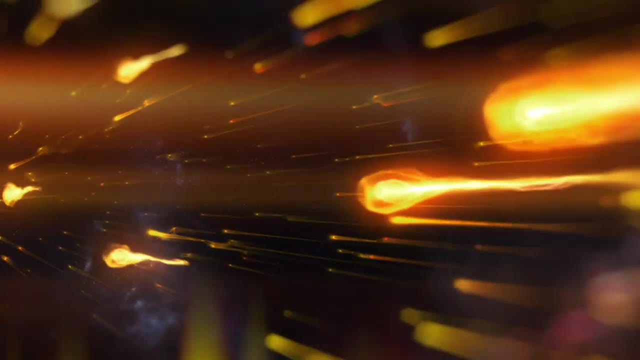 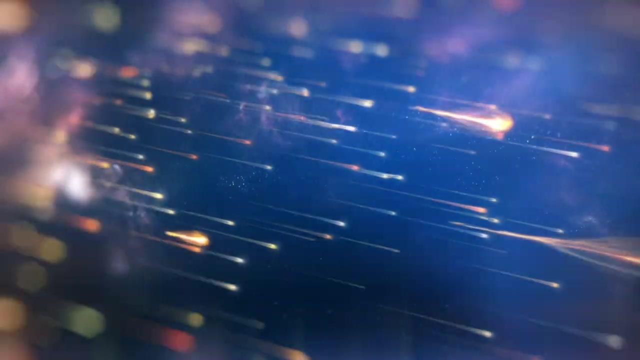 So it sort of runs into it and creates this shock wave and ends up piling up particles at the edge. The shock wave and particles slam together In the collision. the particles steal energy and speed like a baseball accelerating off a bat. The particles transform into something far more powerful. 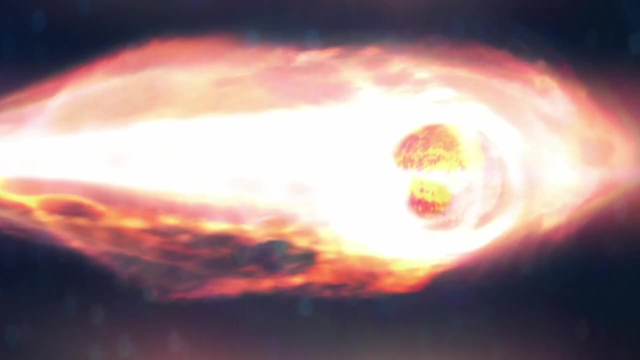 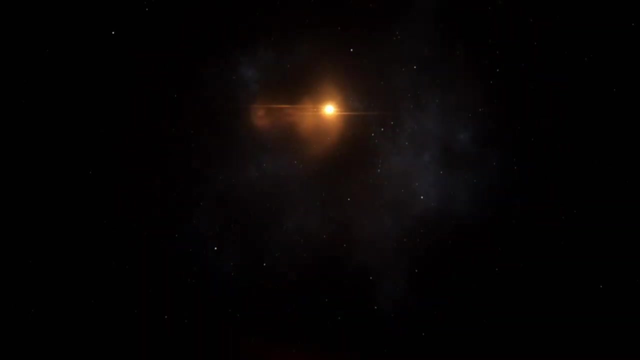 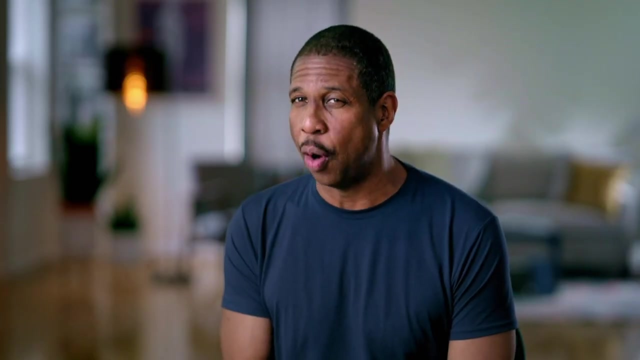 a solar cosmic ray. They're light, but they're moving incredibly fast. The Earth is, on average, 93 million miles away from the Sun And these guys reach us in about an hour. That's 93 million miles an hour. That's pretty fast. 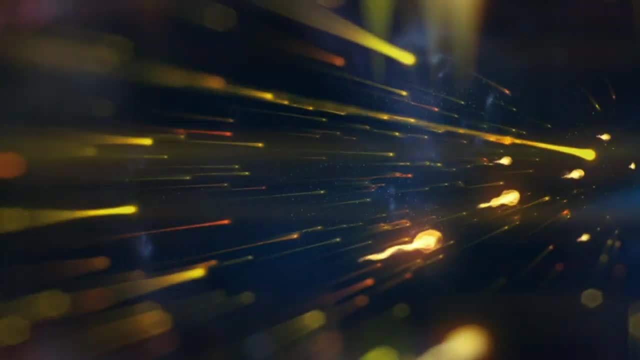 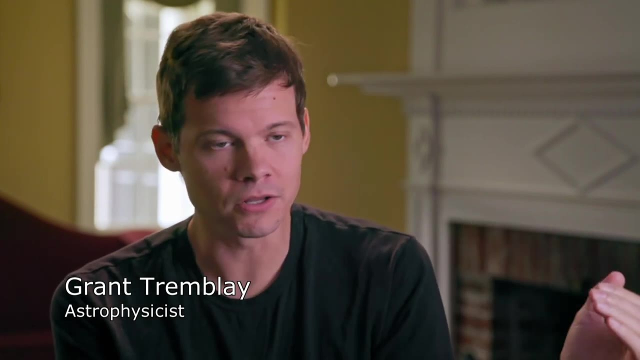 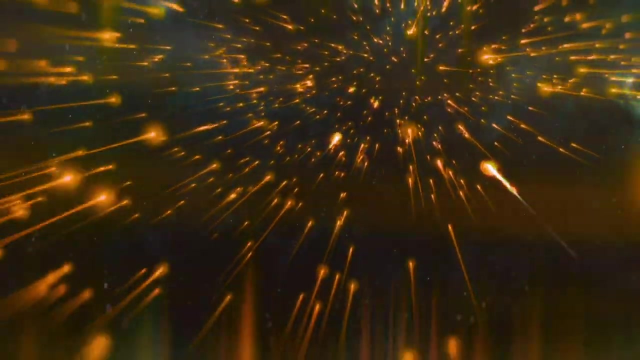 The cosmic rays speed towards Earth. We're under attack. Cosmic rays are by far the most energetic particles that we know to exist in the universe, And when things with very high energy, no matter how small they are, impact something else, they deposit that energy right. 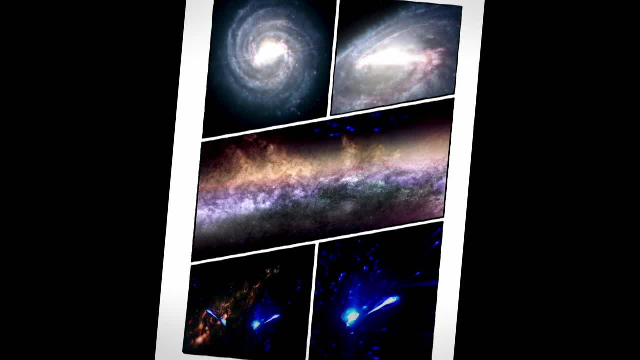 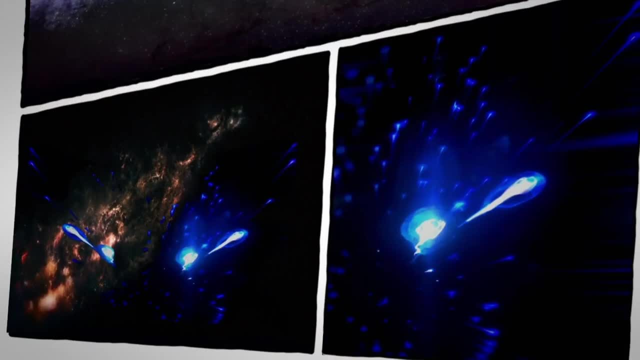 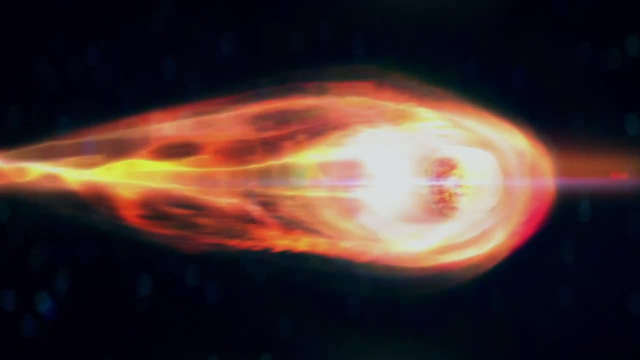 And so cosmic rays can be very dangerous. Solar cosmic rays aren't the only threat we face. Other space bullets arrive from beyond our solar system. There are different kinds of cosmic rays, just like there are different kinds of bullets At the lowest end of the spectrum. are these solar cosmic rays? 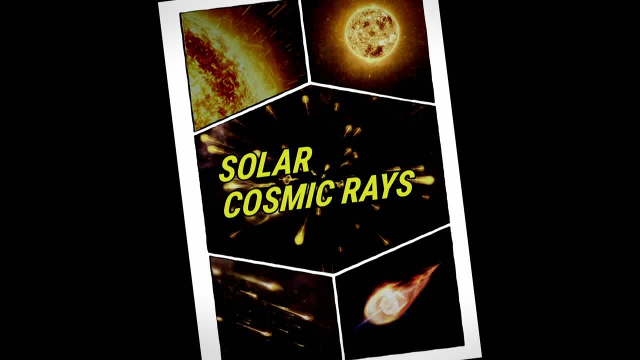 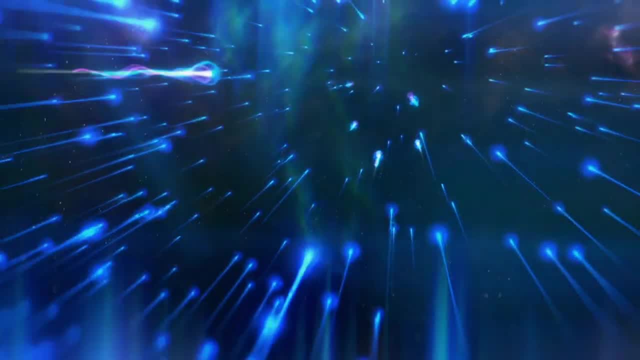 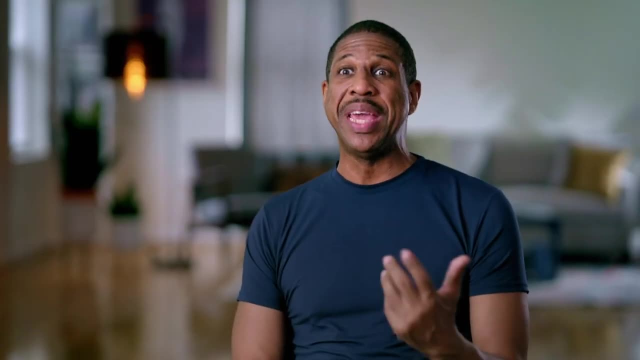 These are like the BBs, and when a BB hits you it might sting for a little bit, but you're not going to get too worried about it. A bigger concern: Galactic cosmic rays. They travel faster and have more energy. If solar rays are like BBs, 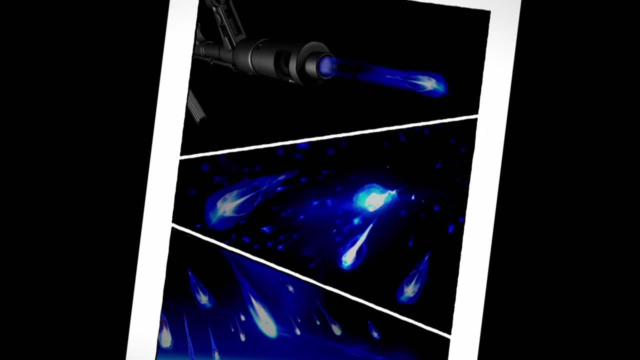 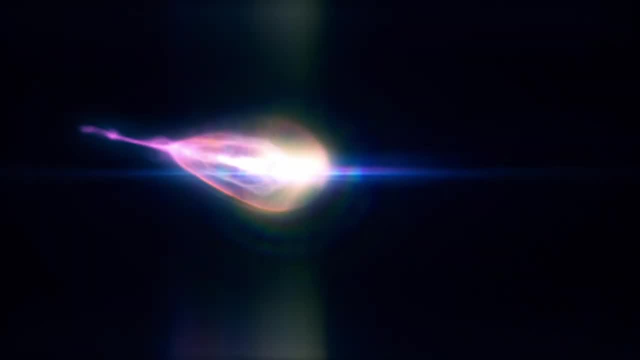 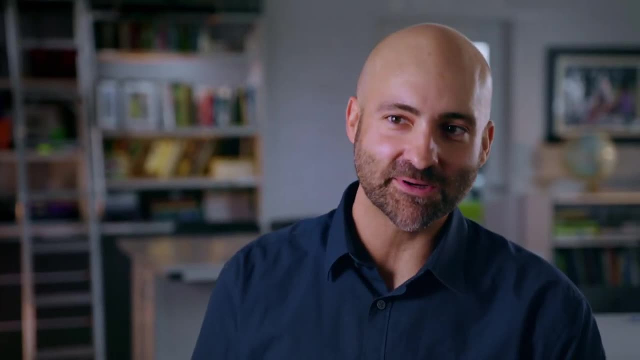 then galactic cosmic rays are like rifle bullets. They're far more dangerous. They're moving a lot faster, but they're also more rare. Faster still are the universe's most wanted ultra high energy cosmic rays. If you thought galactic cosmic rays were bad. 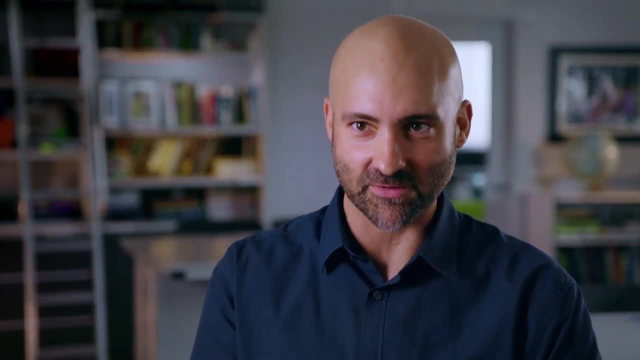 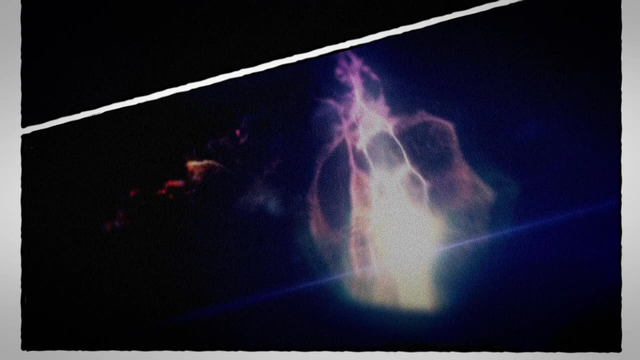 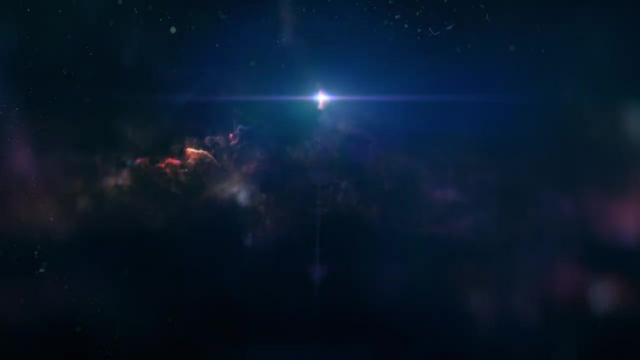 it's because you haven't met an ultra high energy cosmic ray. These are the biggest, baddest, meanest cosmic rays in the universe. These ultra high energy cosmic rays are like hypersonic missiles. They are screaming and they come from the most energetic events in the universe. 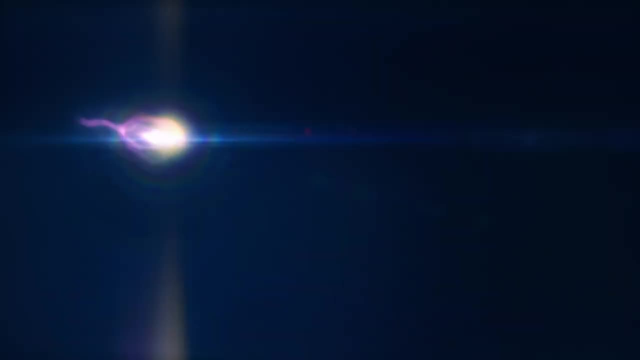 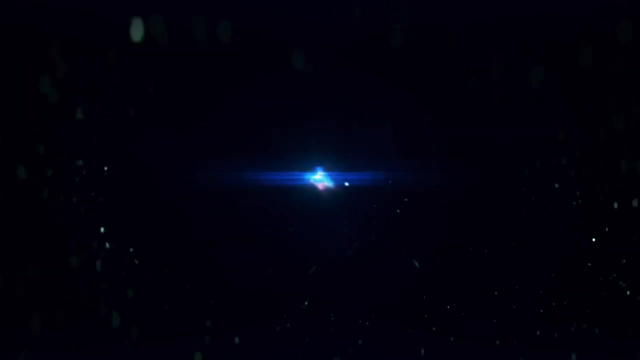 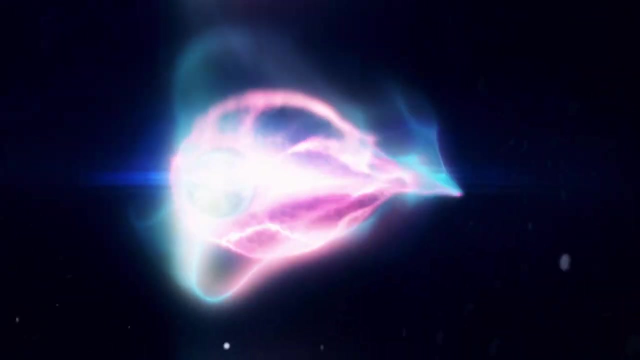 The ultra high energy cosmic missiles are the rarest but also the swiftest. They're almost as fast as a rocket. These cosmic ray particles are moving fast. These mysterious particles are moving incredibly close to the speed of light. I'm not talking about 99% of speed of light. 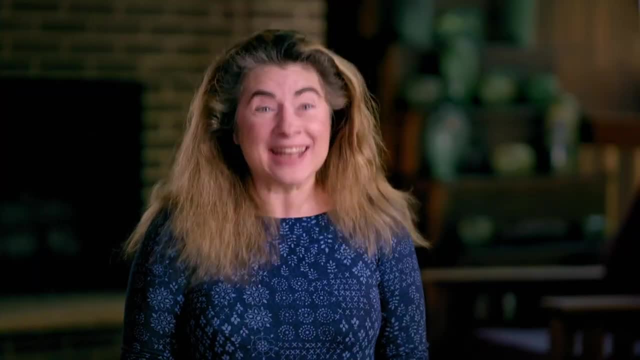 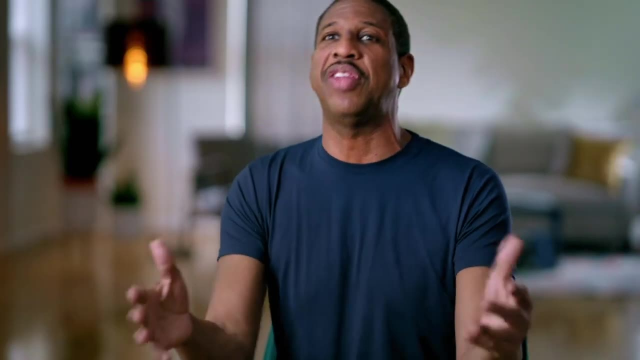 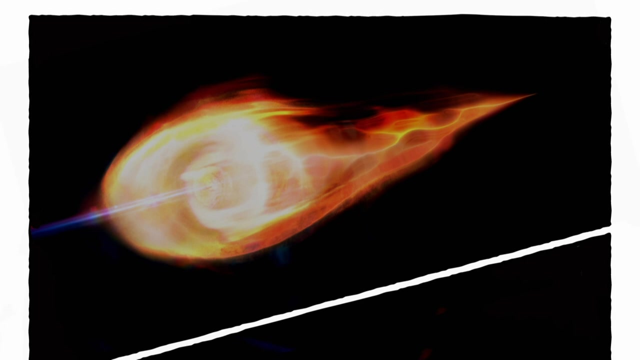 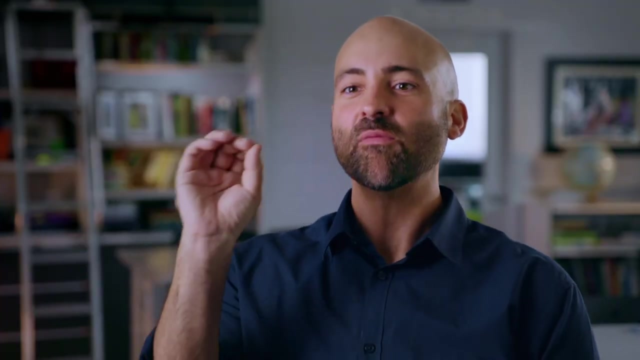 They're moving through space at like 99.999999999999999999999999999999999.. 21 nines, That's fast, That's wild, That's scary. types of cosmic rays are racing through the solar system. If I were to hold up a golf ball in the middle of space, almost 100 cosmic rays pass through. 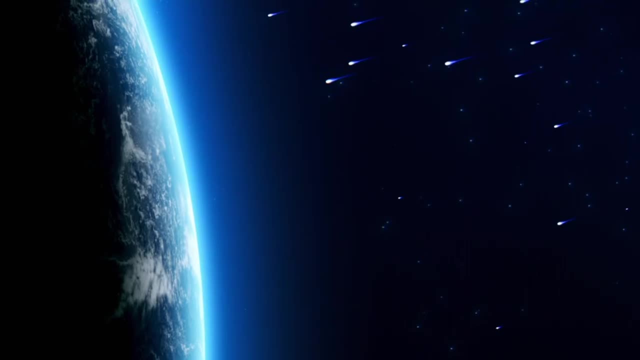 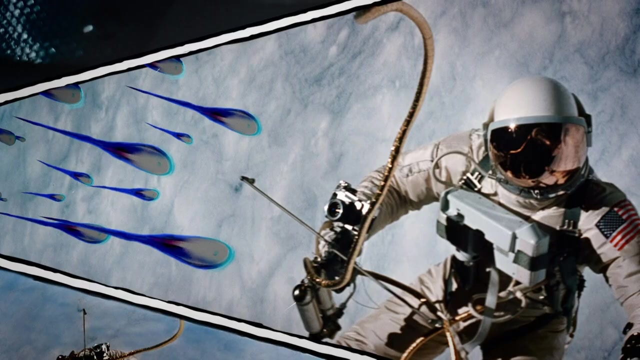 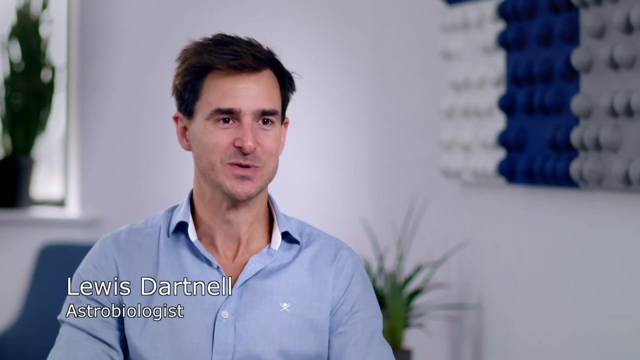 that golf ball. every single second It's a deadly hail of particle bullets, and out in space, our astronauts are caught in the crossfire. Cosmic rays represent one of the greatest dangers for human spaceflight. One of NASA's big goals is to send humans to Mars, and that is a long way away. 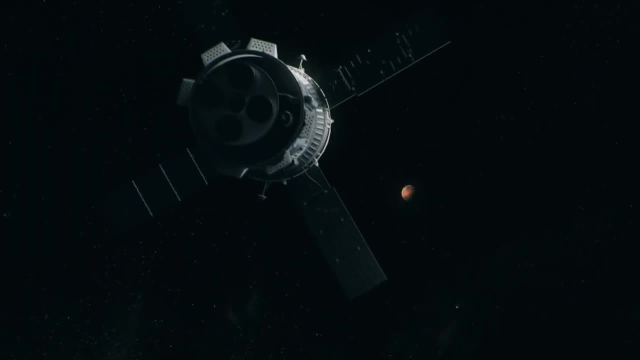 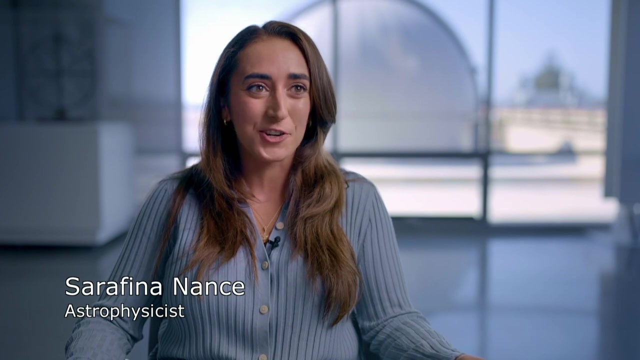 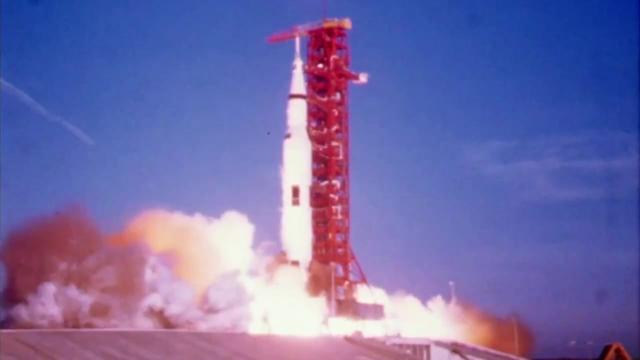 At least a six-month journey and more often about a nine-month journey. That's a big problem. I am hoping that one day I can go to Mars as an astronaut, but I'm definitely afraid of cosmic rays and the more that I read about it, the bigger of a threat it seems. 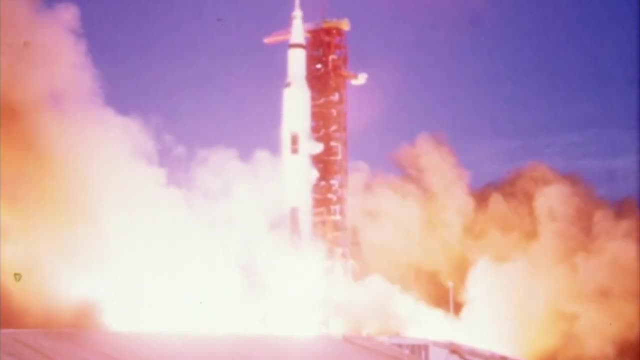 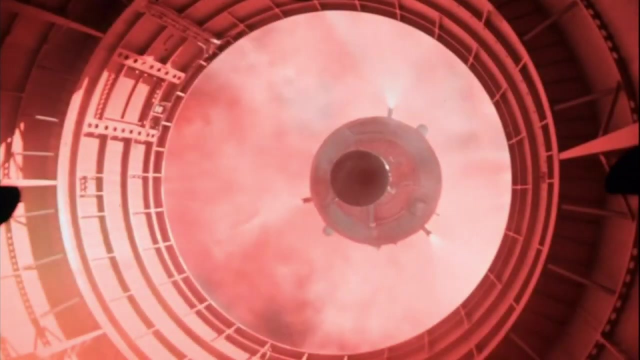 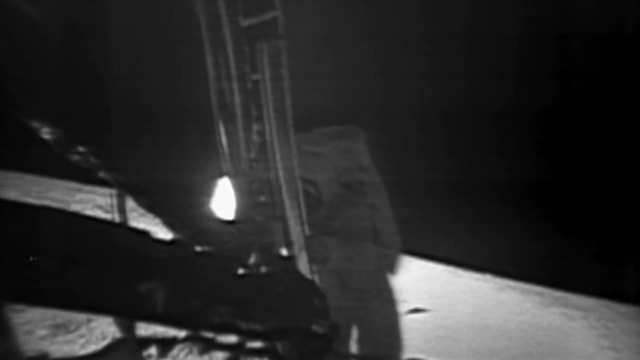 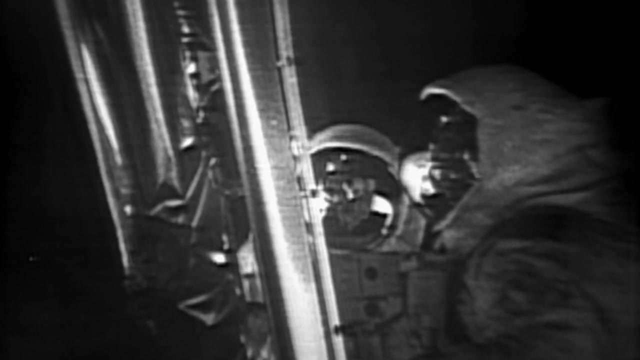 Only one group of people have been exposed to these high levels of cosmic rays: The crew members of the Apollo missions, July 1969.. That's one small step for man, one giant leap for mankind. One of the astronauts, Buzz Aldrin, sees something strange. 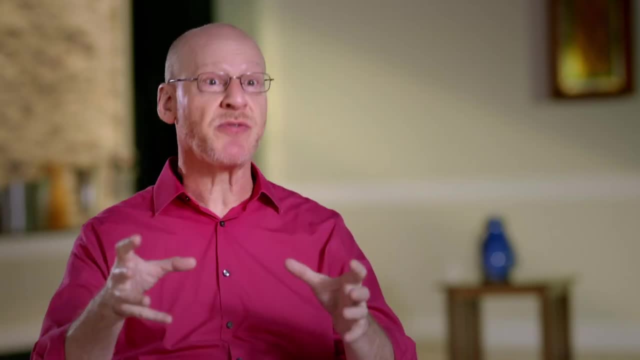 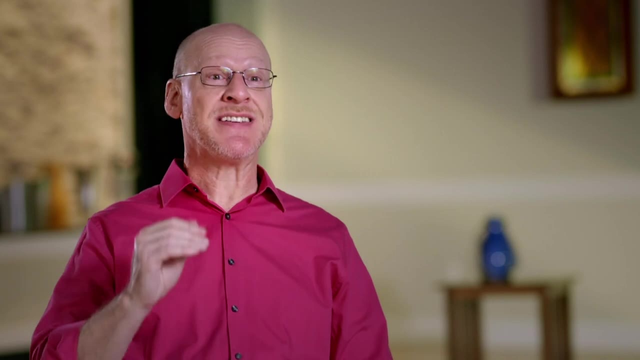 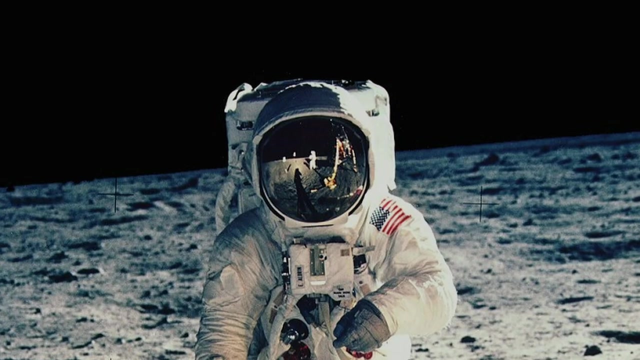 During Apollo 11, Buzz Aldrin reported seeing tiny little flashes- sometimes That's right- When he was looking around. That's pretty weird, but what's weirder is that he saw them when his eyes were closed. Later missions also report seeing odd flashes of light. 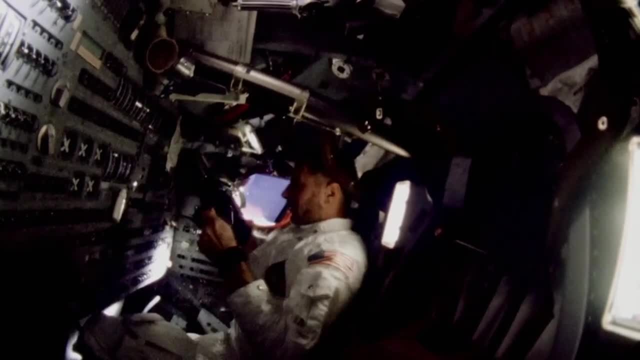 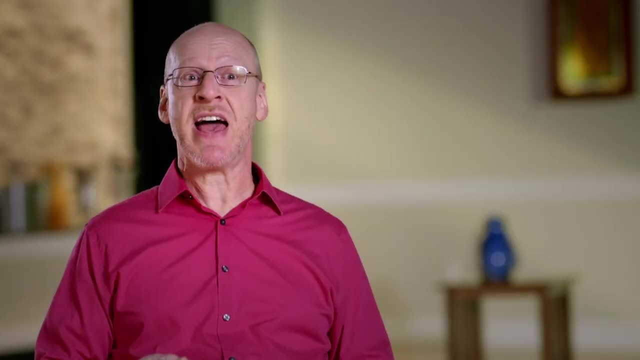 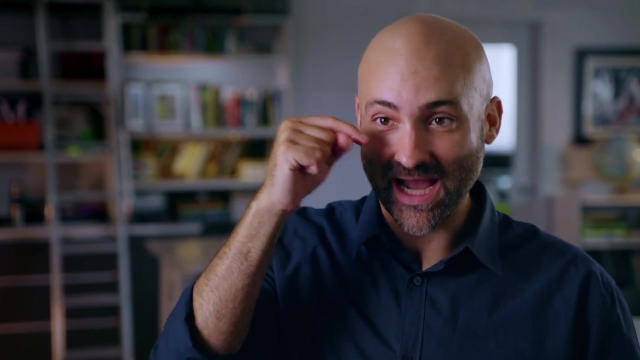 The astronauts describe the flashes as spots, streaks and clouds. Apollo 15 Commander David Scott reported seeing one that was blue with a white cast. The astronauts also report seeing a blue diamond. What's happening is that a cosmic ray is entering the eyeball and then striking molecules. 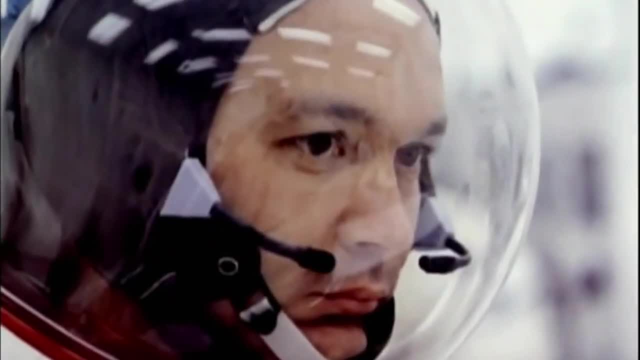 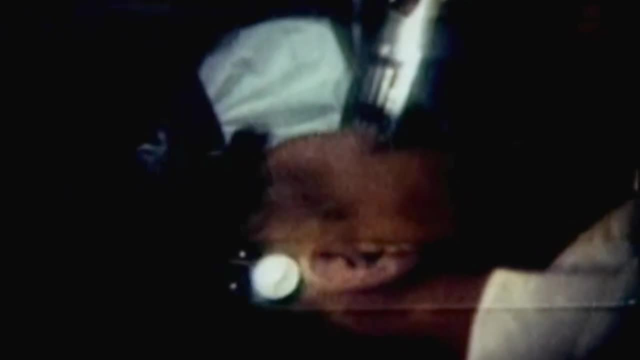 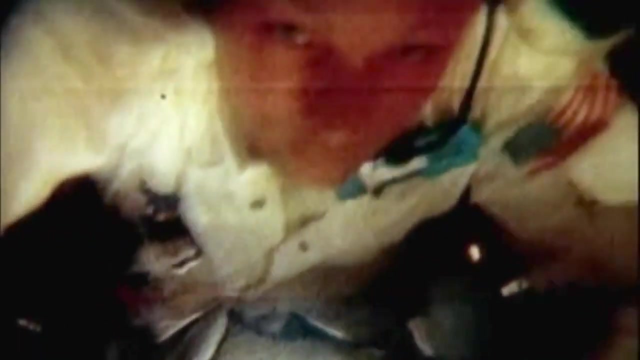 and giving off a flash of light. An alternative theory is that it triggers the layer of sensitive cells in your retina, So you perceive a streak of light even though no light ever actually existed. The cosmic rays cause long-term damage. Inside of the eye's lens there are these fiber cells that are transparent. 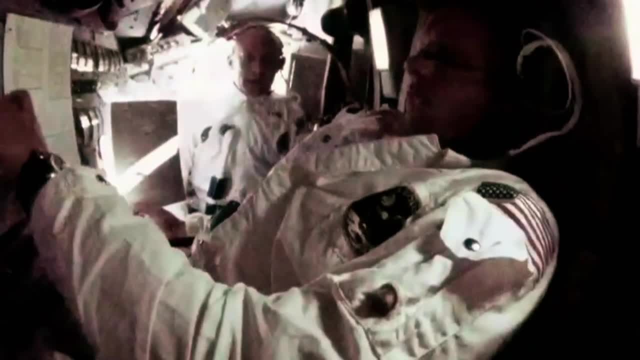 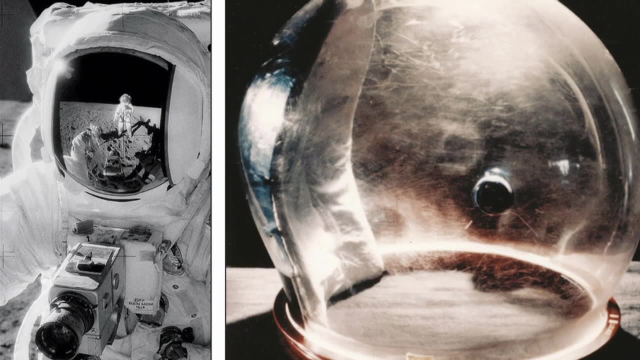 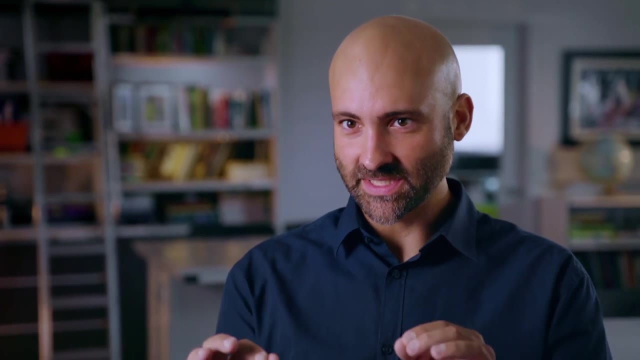 Well, when a cosmic ray travels through them, it can damage those cells and make them cloudy, causing cataracts. When NASA examines the astronauts' helmets, they find tiny tracks etched through them, Evidence of cosmic ray impacts. When we say that cosmic rays are like tiny little bullets, we're not joking around. 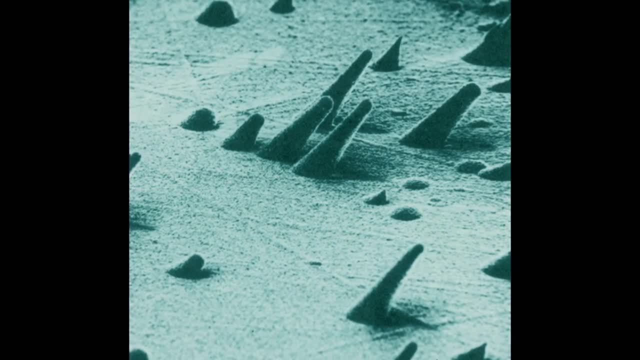 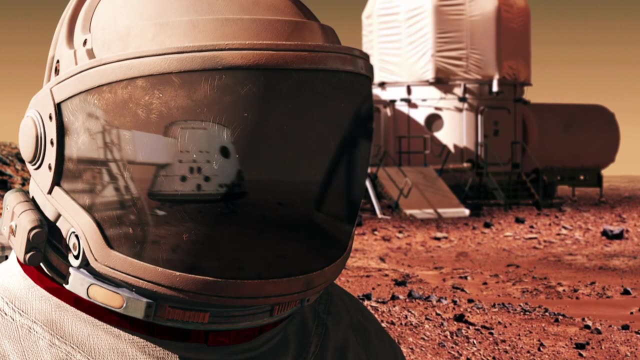 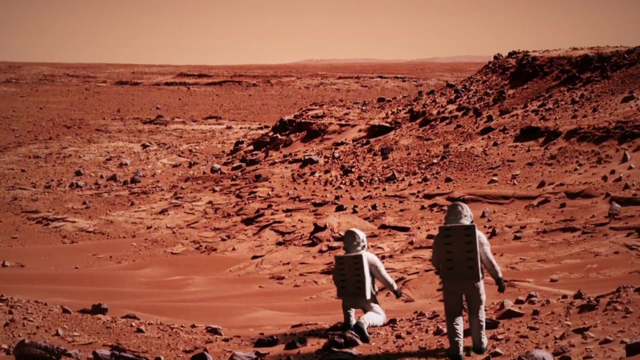 In some of these, burrowed all the way through the helmet, Which means it ended up in the astronaut's brain, which just makes me feel weird to think about. What might that long-term radiation do to your brain, to your ability to reason and